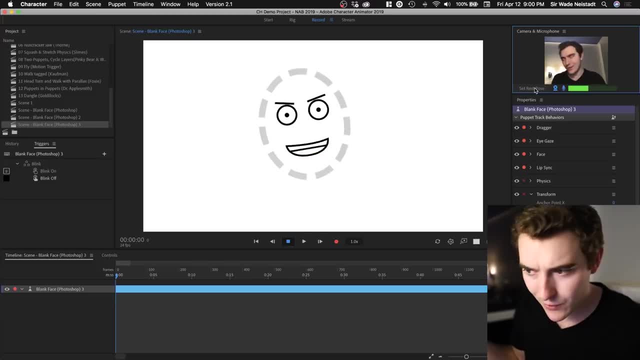 So if we look at the screen, my webcam is actually controlling this character. I can look around, I can do things with my eyes. I can go ha ha, ha ha, evil, But you can see, it'll track my head motion, it'll track my eye direction. it'll do things with my eyebrows, my mouth. It'll try its best to figure. 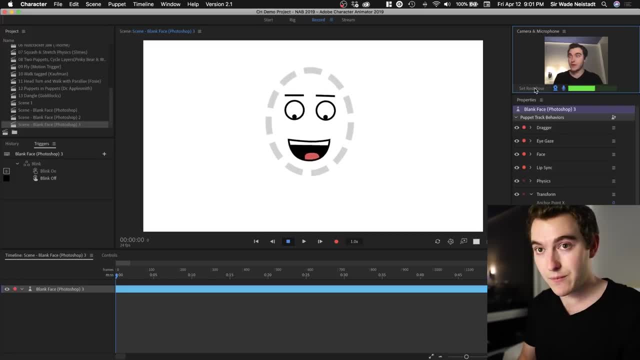 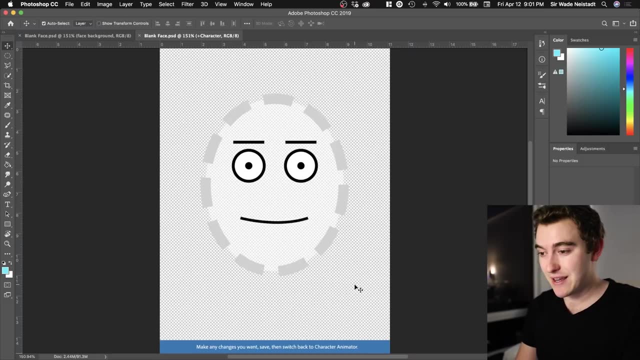 out the words I'm saying and give you the lip sync for the voice and what your mouth is doing. So this is the actual puppet and there's an entire rigging system, which is a lot easier than 3D rigging in my opinion. But the cool thing is if I just jump back to Photoshop and make any change. 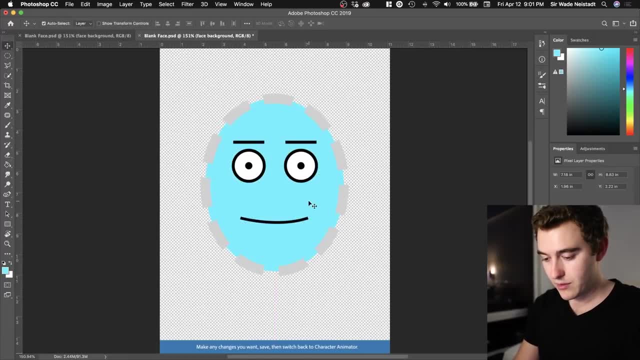 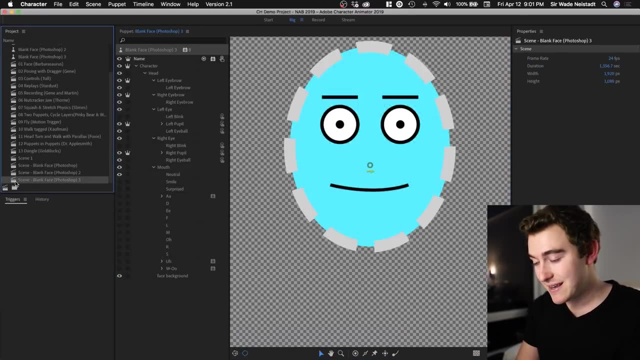 I'm just going to take the background layer, I'm going to turn it blue, call it good and hit save. I'm going to jump back. It'll automatically update the puppet here in Character Animator And if I jump back into my scene, it's immediate. You can make these changes really quickly and 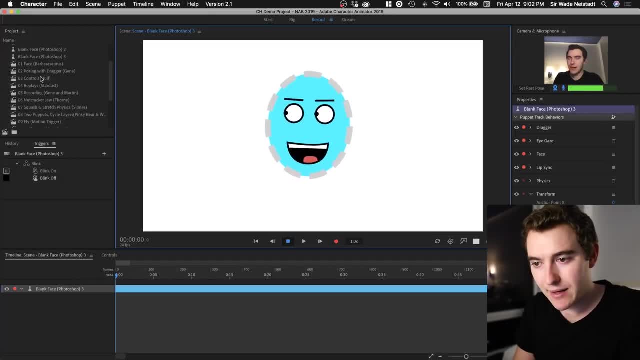 customize your characters, but we're just looking at a face and that's not super helpful, So let's go ahead and do something more interesting. So if I open Tull the Cat, this character here in the top left corner, you have your projects, where you keep your assets, your puppets and your 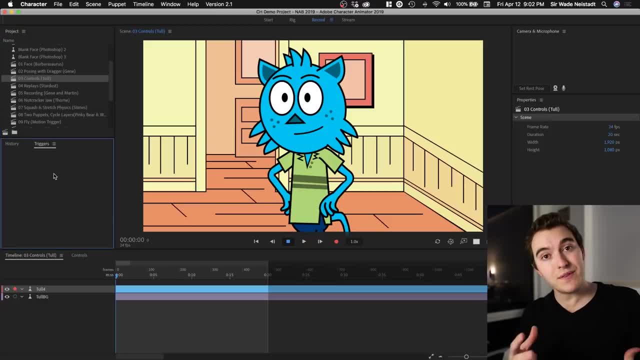 scenes, your actors and your sets Under. that are your triggers, which are different things that you can control. So if you had a button on your keyboard or other things we'll talk about later, it can actually trigger animations or facial expressions or motions with the arms or different. 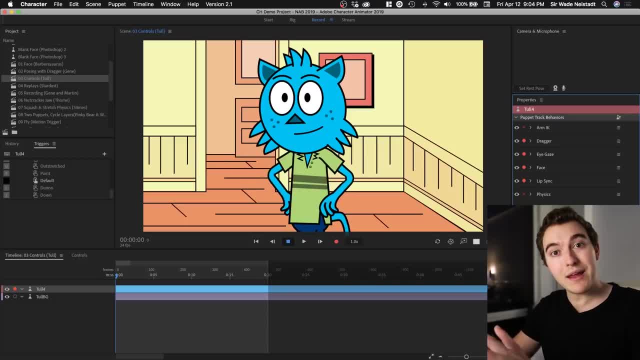 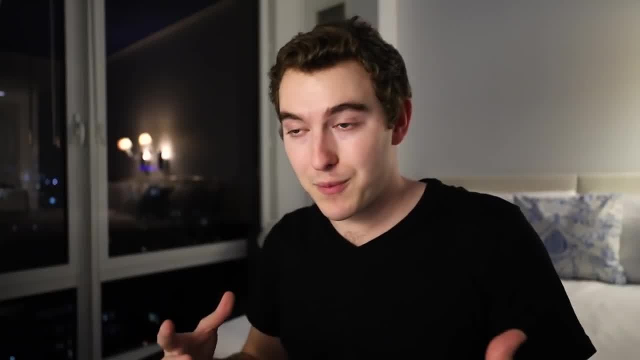 things that you can build into your characters and just kind of pre-make everything. so it's all ready to go. You pretty much just pick the character you want to activate, you hit play and it'll start recording. You do all your acting and your performance and you can hit all the buttons. 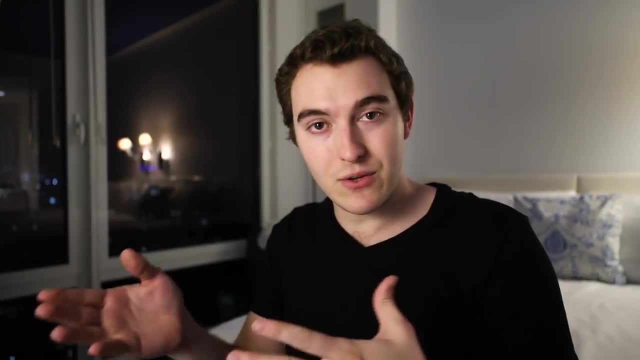 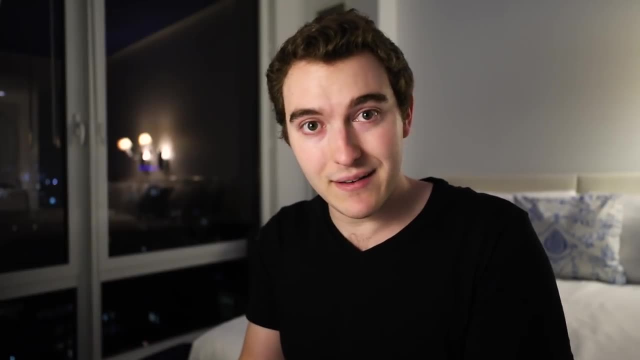 you can trigger different motions and it will save all that as you go and then you can tweak it later or export it right from there. So it's real-time animation on a really interesting level. that gives you a lot of flexibility to make cool stuff very quickly. In the top right corner is your camera and microphone, If you have. 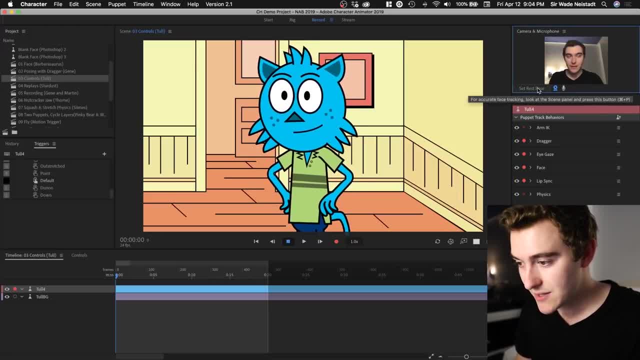 these turned on and you have a webcam. what I'll do is I'll look at the character and I'll say set, rest, pose. with a blank facial expression. That resets the character to match me and if I turn on the microphone, you can see that he begins to mimic my face shapes. If you don't like the way, 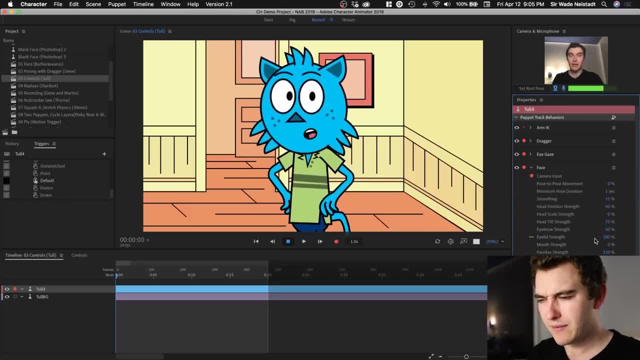 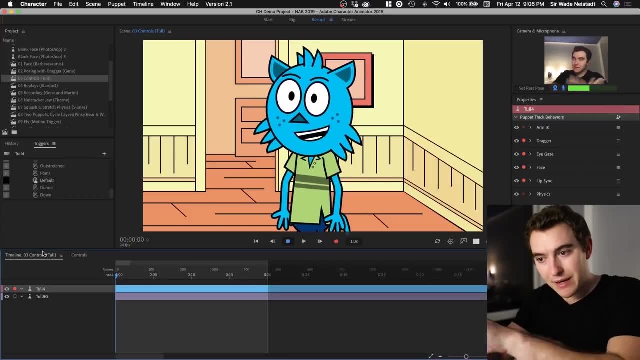 that this is happening. there are settings you can mess with, Like: if these eyebrows are not enough for me, I can dial up the eyebrow strength. I can get them a lot more aggressive. Now I know that at first class this might look a little complicated, It might look a little bit. 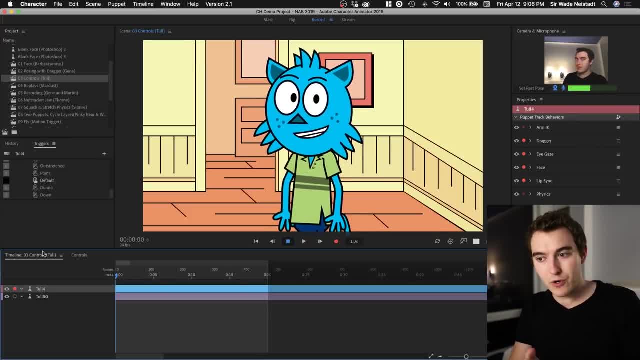 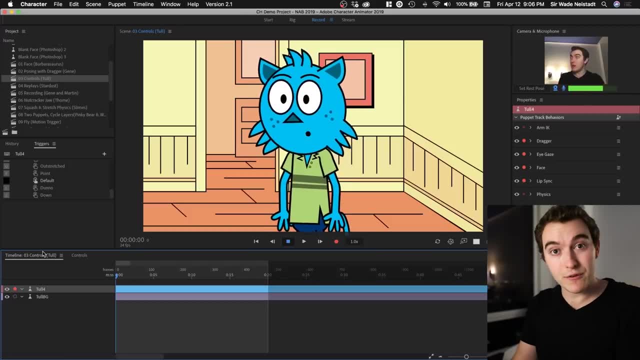 like After Effects or Premiere or a program that, when you haven't messed with it before, you look and you go, oh, this looks like a lot. Well, believe me, it's really not. It looks complicated at first just because it's a new interface, and that always happens when you're 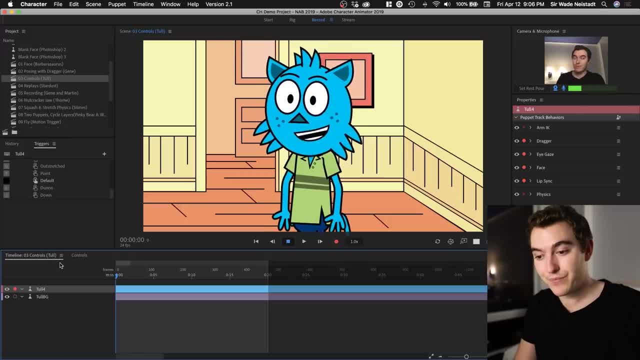 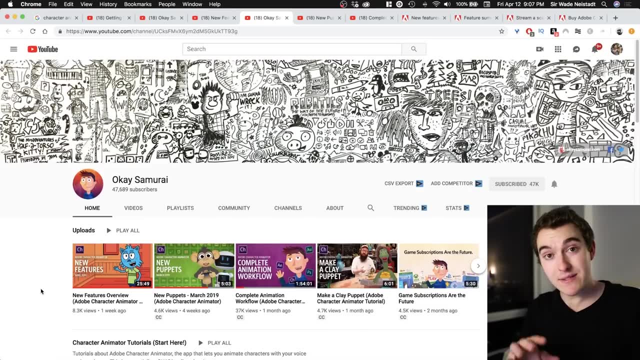 learning new software, But this is actually a really simple program to get used to, And if you want to learn it, let me just first of all point you to the best learning resource for learning Adobe Character Animator, and that is the YouTube channel OK Samurai. This is managed by Dave Werner. 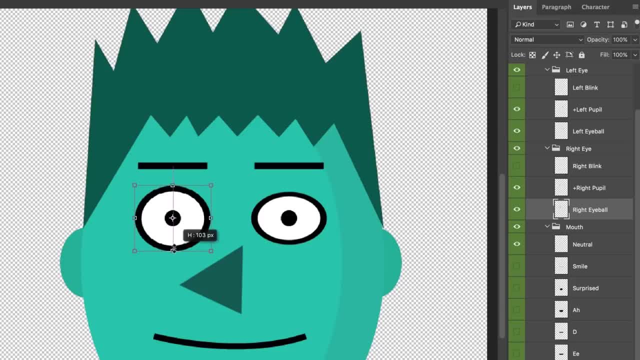 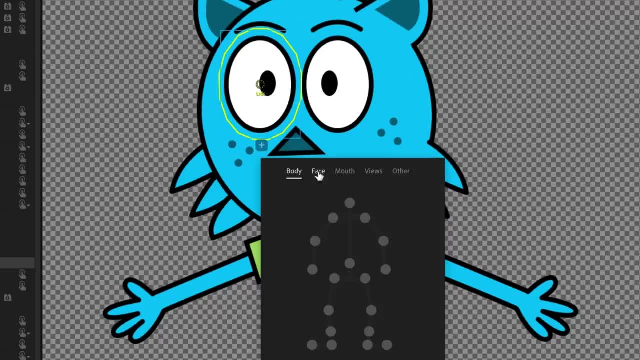 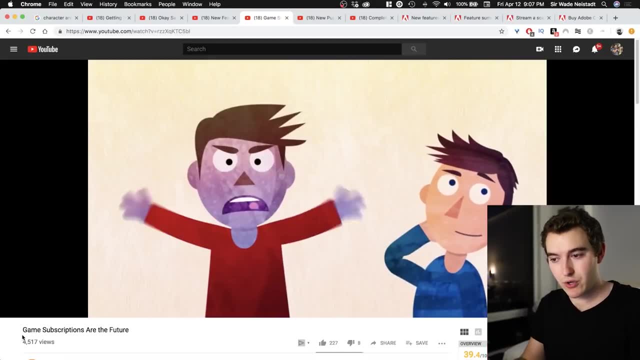 greatest tutorials on Character Animator. Whenever I need to learn how to do something in the software, I just go watch his tutorials. They're really good. He's great And just to give you an idea, this is one of the videos that he made And I just wanted to show you these types of 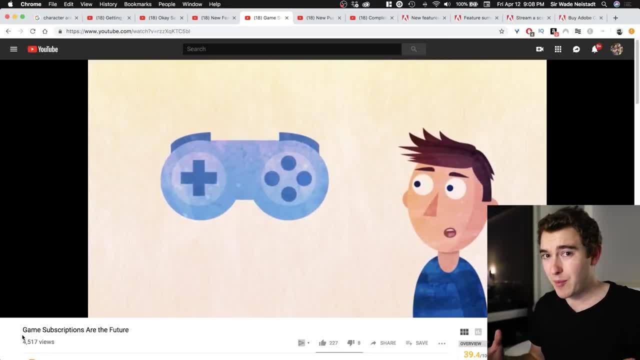 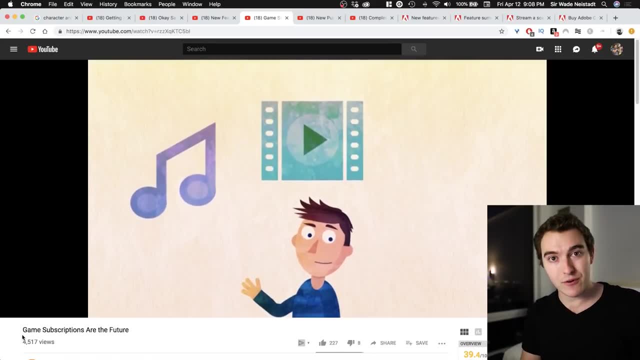 explainer videos that you see a lot of businesses and like corporate stuff. People pay a lot of money for these types of videos and you can make them really quickly and really easily with Adobe Character Animator, versus trying to do it in After Effects, which I've done. I've done freelance. 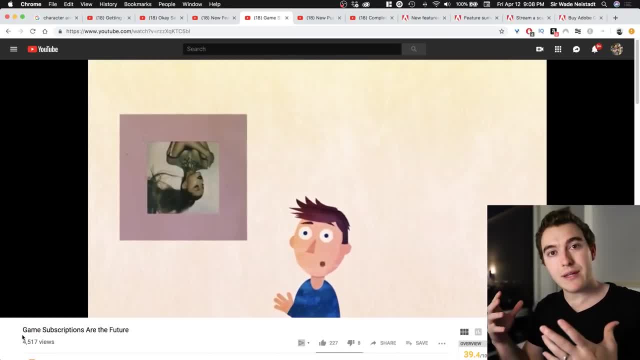 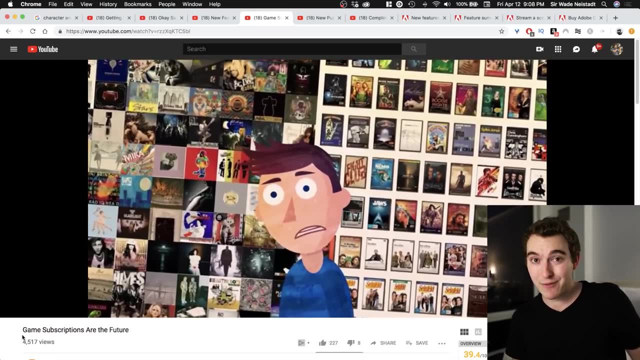 using After Effects, where I'm putting puppet tools and I'm manually animating these things by myself hand keying them in After Effects. This is way faster and I have switched my workflow to using After Effects for those kinds of videos to using Character Animator for all the character. 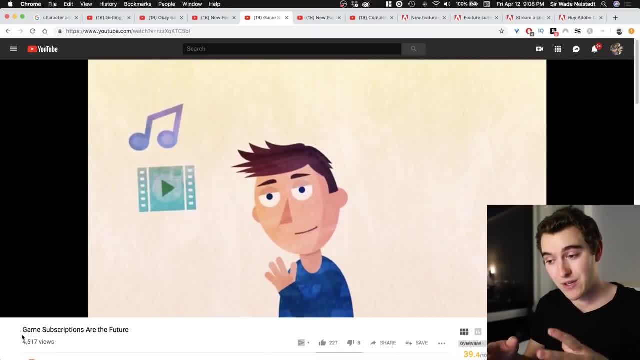 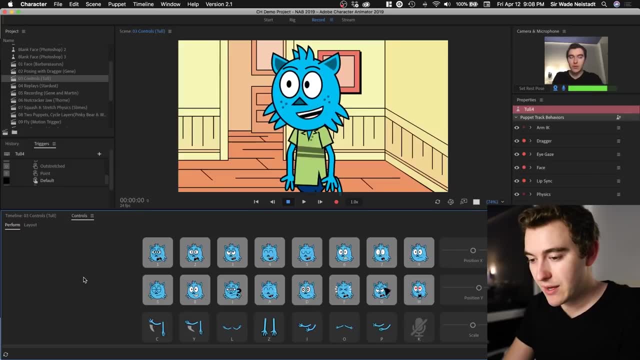 based stuff and then I'll do extra compositing things in After Effects So you can actually make a lot of money by using this tool, just so you know. But jumping back in, you can actually have a controls thing setup so you can hit buttons and get a more suspicious expression, or he's a little. 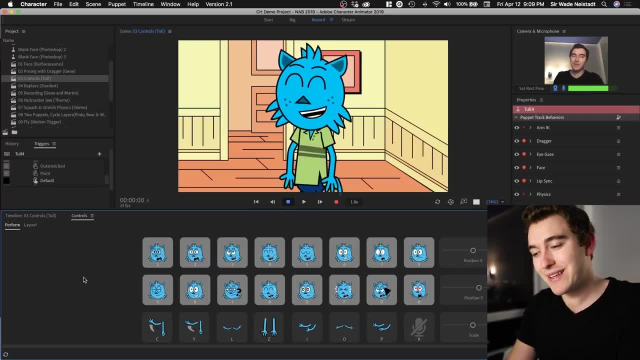 bit more alert. He's a little bit more alert, but he's a little bit more alert. and he's a little bit more alert or very laid back hanging out and ah, he's really happy about this, But oh no. 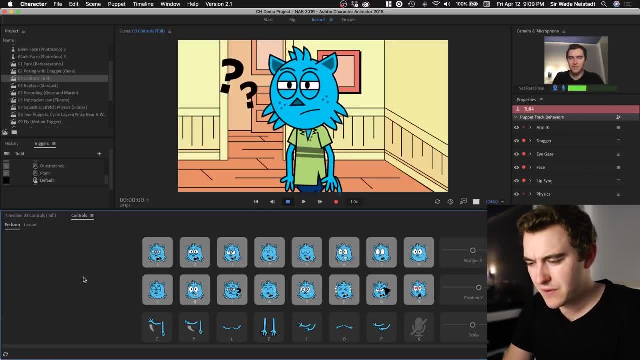 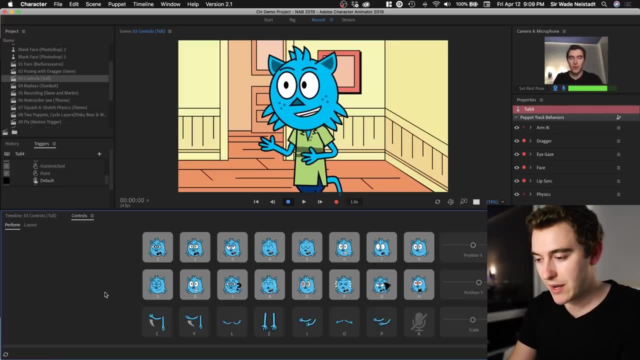 what is that we see? Oh, I'm completely terrified. In fact, I'm confused. happy, Oh my gosh, it's so beautiful And upsetting at the same time. But now, wow, Gesture over. this way you can have him do the different faces at the same time. What the heck is that? But you kind, 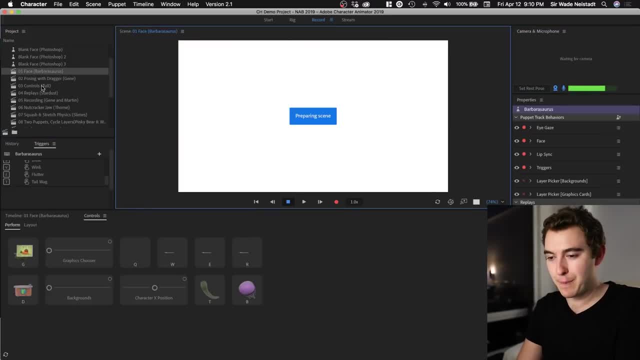 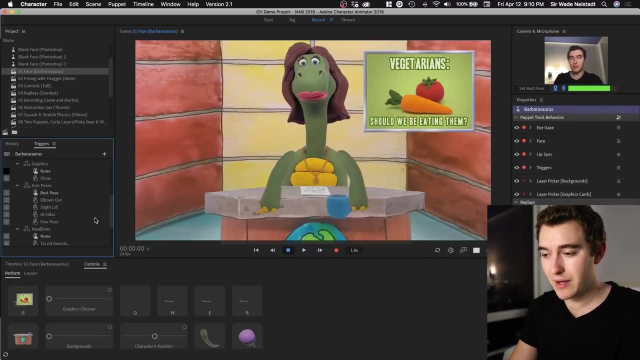 of get the gist Now quickly, I'd like to just jump over to a different character to show you a different style. This is a news anchor dinosaur made of clay. This is an actual stop motion puppet. You can have her grab things. You can hold the pencil, You can hold the mug. 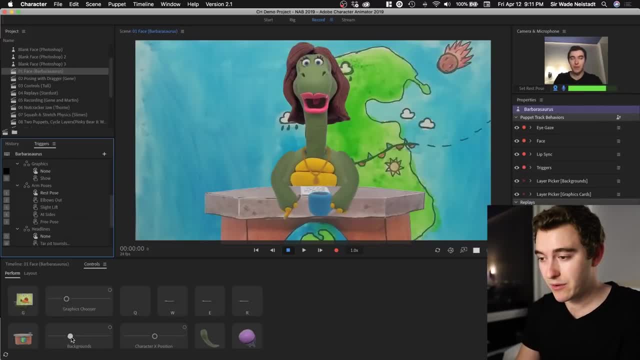 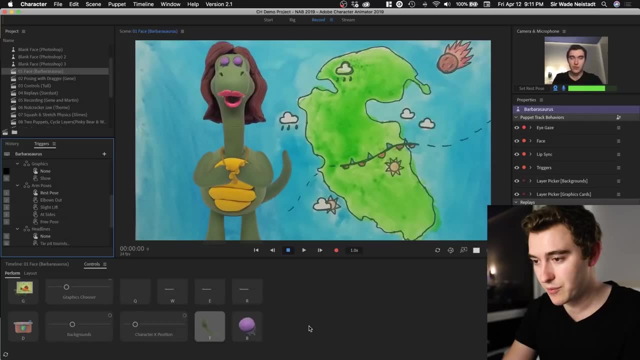 You can switch the graphics. You can have an entire show. We can switch the background to be more of a weather background. We can turn off the table, move over here, have her gesturing, doing all this kinds of stuff. You can control the blinking. We can put some breaking news on. 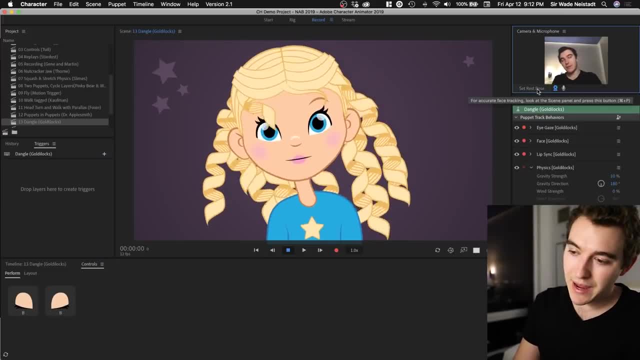 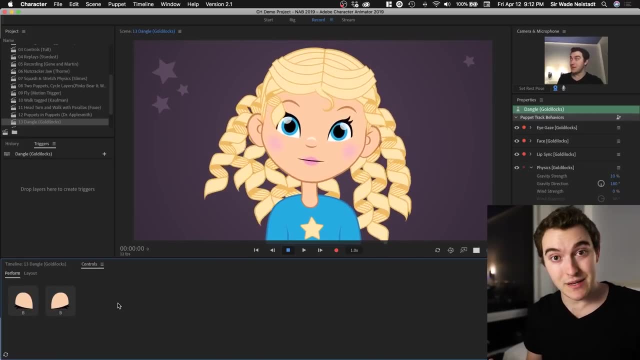 the stage that there are tar pit tourists reported missing. You can have overlapping action built into your characters. There's physics engines, There's all kinds of like insane stuff in here And, in my opinion, not enough people are exploring the possibilities of using this tool for tons of. 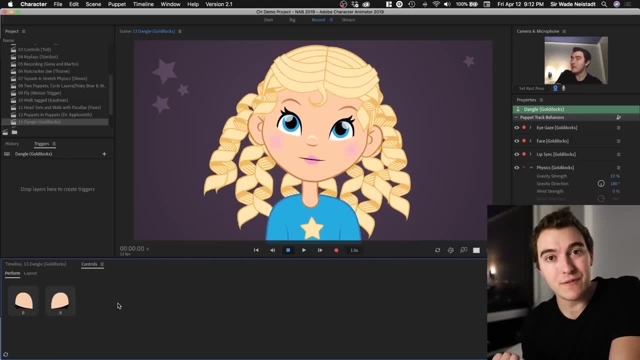 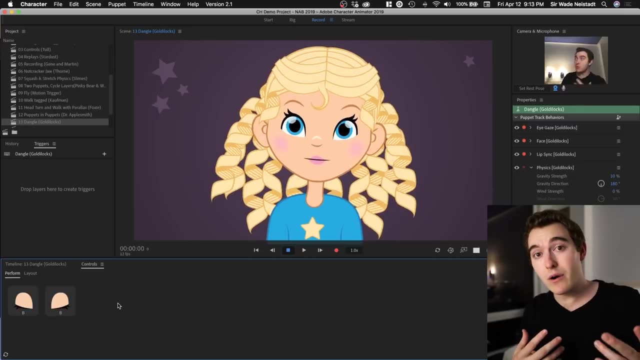 stuff. For example, something that I'm personally really excited about, one of the new features is Twitch extension. You can actually stream on Twitch using these characters or whatever character you want. So if you are camera shy and you want to have a YouTube channel, or if you are 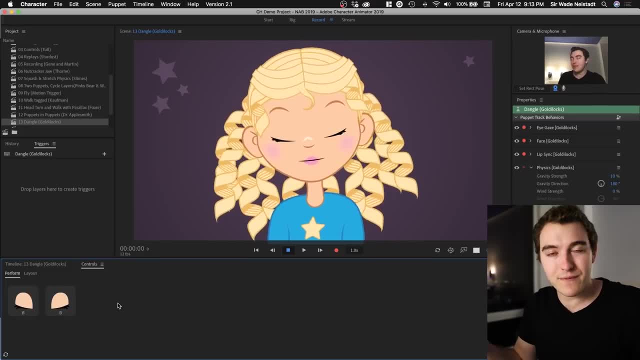 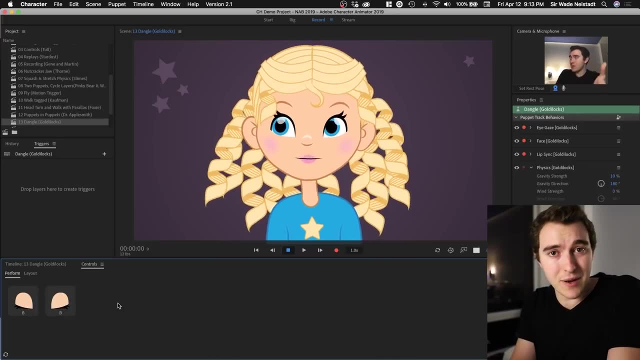 camera shy and you want to do Twitch and maybe you don't have the best setup and you, I don't know, for some reason you don't like being on camera, but you want to be on Twitch or YouTube or whatever. you could do it. this way You could get a character made of yourself or of anything else. some green. 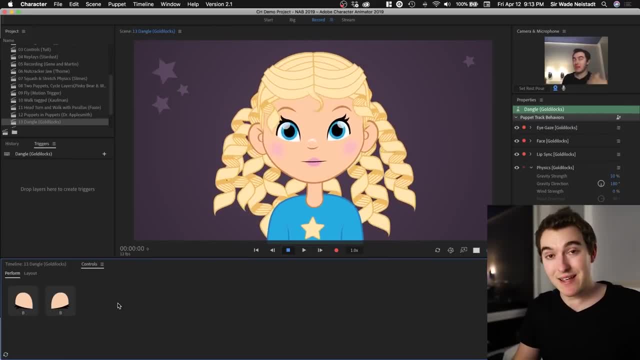 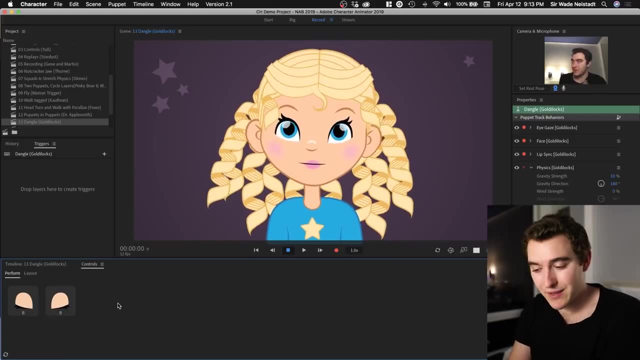 alien who knows. You can set up different animations. You can have the hands do different things. And another cool thing on Twitch- this is something I'll be setting up very soon for my channel, if you want to join on Twitch is when viewers give bits or different things they can. 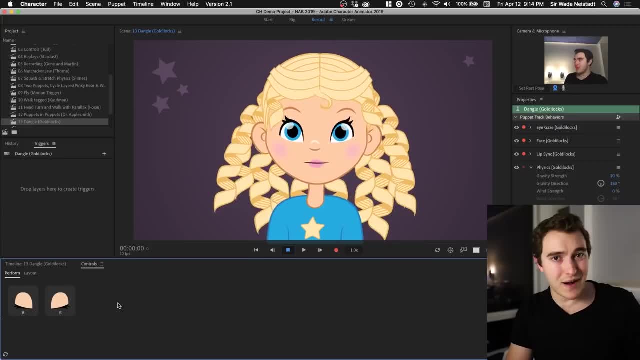 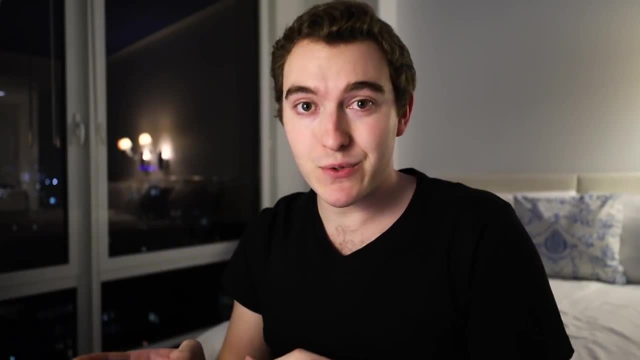 actually trigger different animations If they want to make you laugh or cry or smile or dance or run around in circles or whatever it might be. the audience can actually control your character in different ways that you can set up And, if you remember, I actually used this tool to make this. 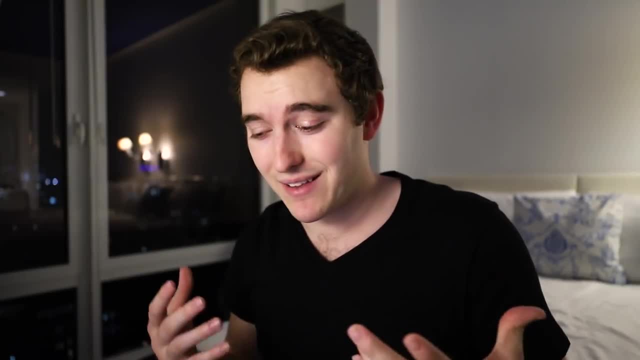 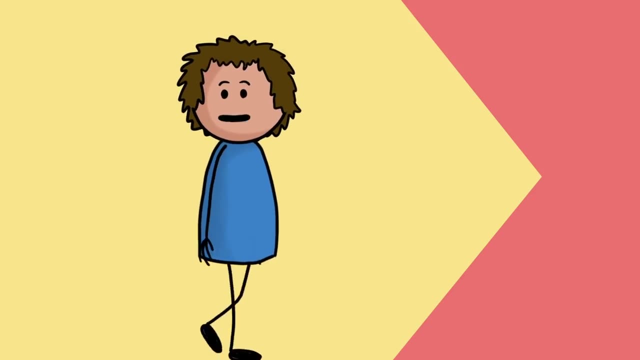 CTN video I needed to talk about, you know, ticket information and a lot of dense topics that were not very exciting for like five minutes straight, And so, rather than trying to put a bunch of graphics on screen or to try and just hope you stick around looking at my face the whole time, 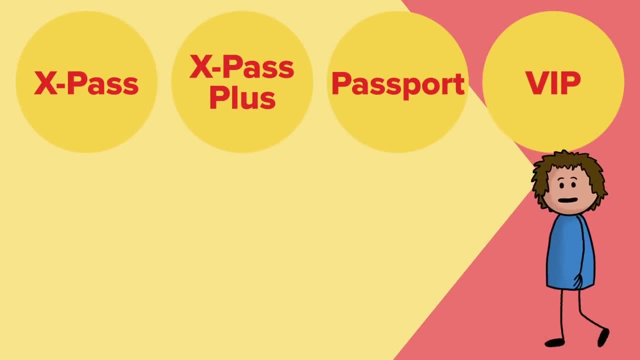 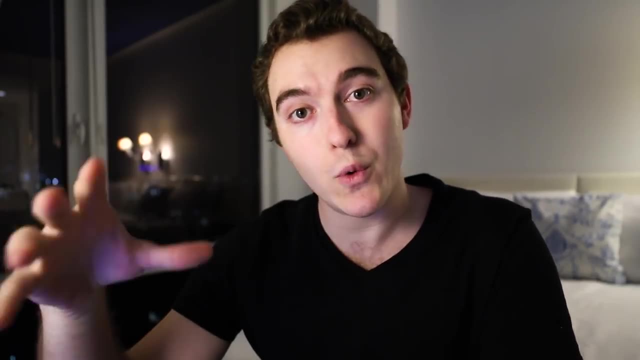 I decided to use Character Animator to put a stick figure walking around the screen and pointing at things, And I just recorded the animation. It was much, much easier and it was a lot more fun to watch, in my opinion, than watching me talk. This is a great option for those of you who want to try 2D animation. 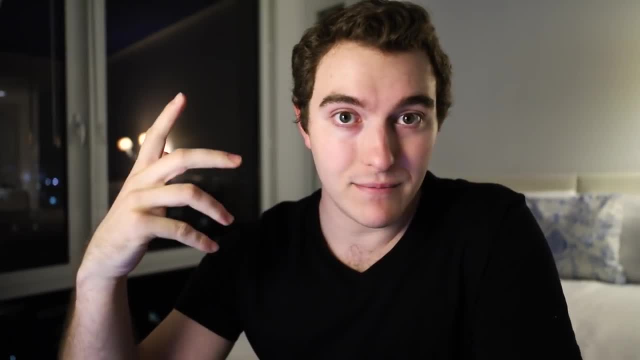 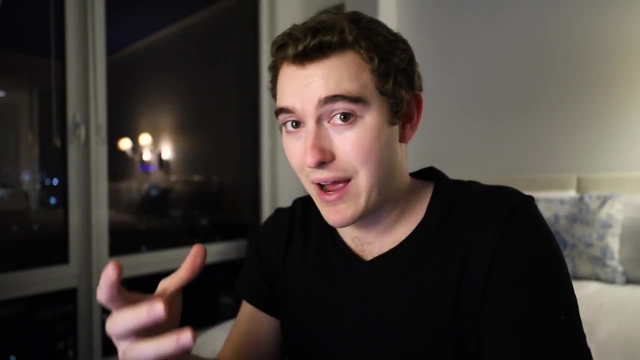 but don't know how to draw or aren't necessarily the best at. you know manual puppet animation in After Effects, If you have a show that you've been wanting to make or an animation that you've been wanting to do in 2D, but you haven't figured out how to get the skills for it. 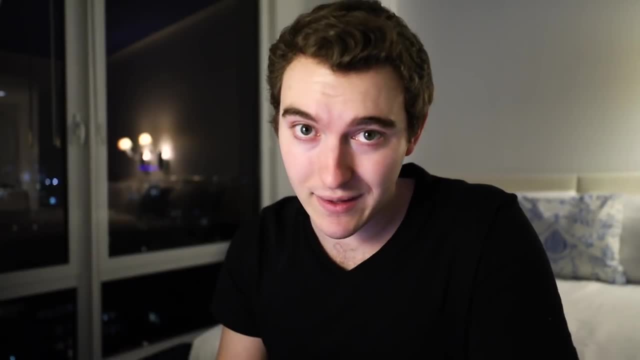 this is a great thing to get started. It makes something really awesome very quickly. One last thing: if you want to make yourself in this program but you don't have any skills in Photoshop to like build yourself, they have a thing called Characterizer. 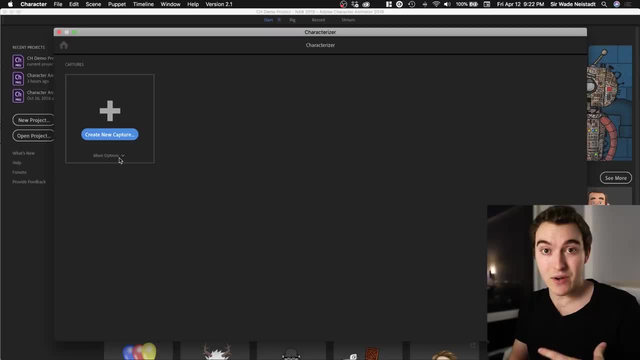 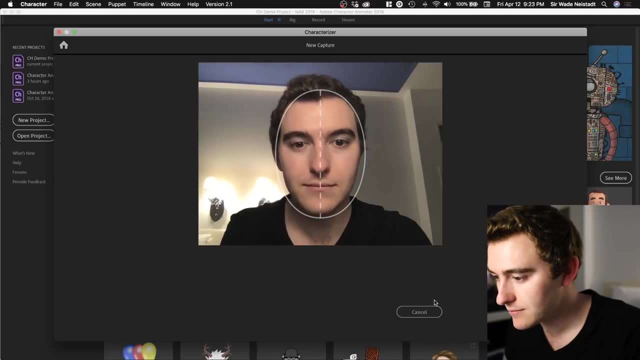 which is a way to capture yourself through the webcam, and it'll stylize it in various ways. Smile in three, two, one. Repeat after me: Photoshop, Photoshop, Woo-hoo, Woo-hoo. Okay, so that was interesting. I haven't done that before, actually. 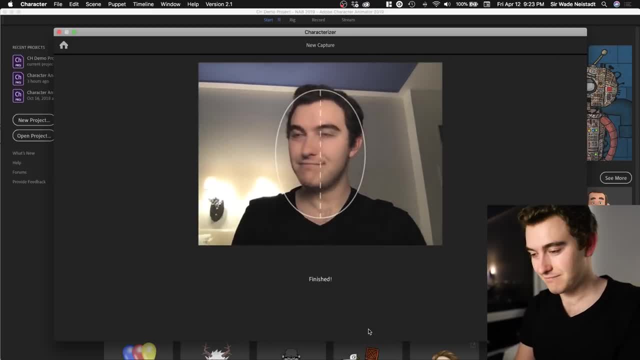 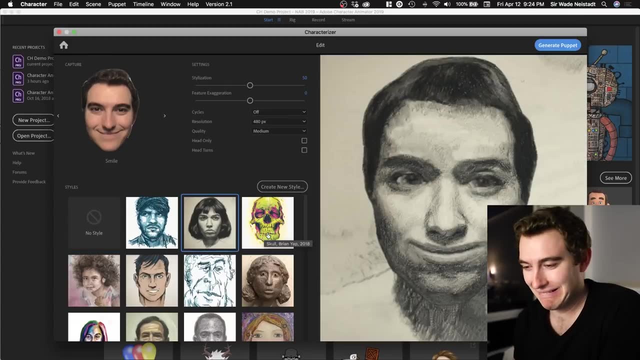 So let's hit. continue. Great job. Your Characterizer capture is now being created, So this is the first time I've actually done this. Let's see what happens. Ooh, Ooh, Ooh, Ooh. This makes me look like a ghoul from Fallout. I just gotta change the colors. 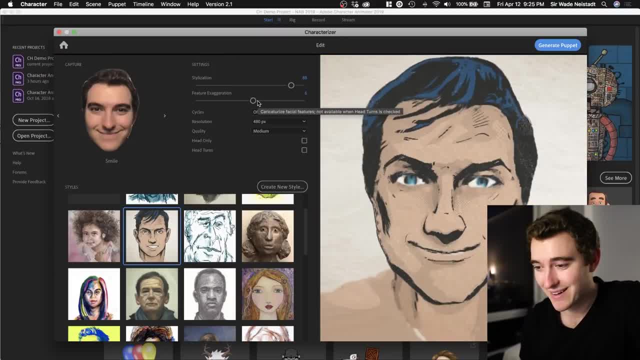 Weird, weird, weird, weird. This one makes me look like a superhero. I kind of like this one. Oh, it made me into like a Wookiee dog person. Okay well, this just got a whole lot more interesting. 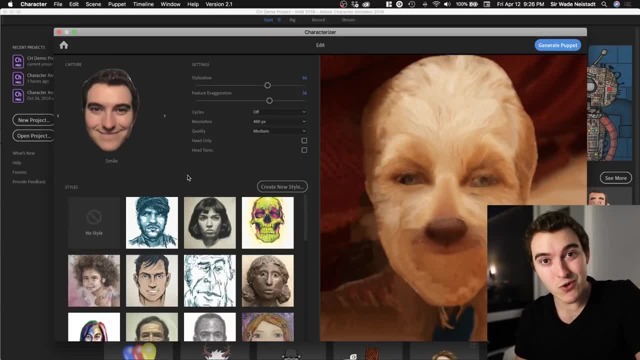 I say: we explore together, make something cool. hashtag it with character animator if you post it somewhere, so that the team at Adobe sees it. and tag me in anything you make, because I'm super interested to see what kind of crazy stuff you guys come up with. 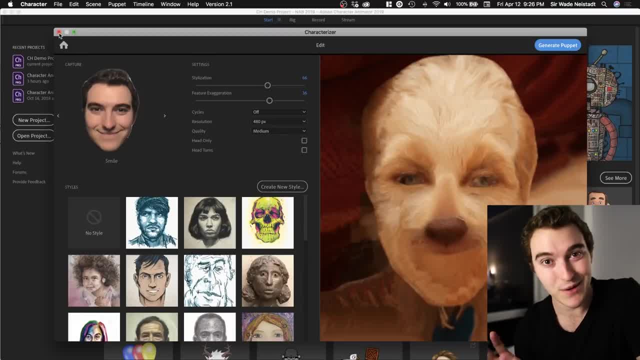 Because I love seeing what you guys make, and I feel like you're gonna make some wild things with this tool. I hope you enjoyed this video. Now, before you click away, give me one second before you leave. I have an announcement to make. 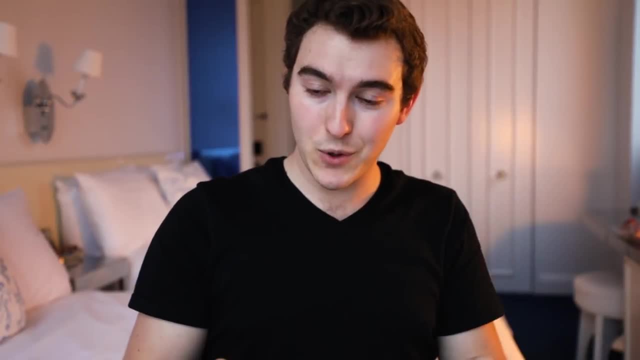 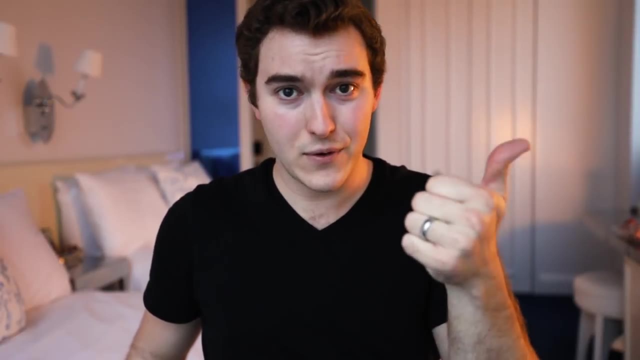 We, as of this moment when I'm filming this video, are 37 people away from hitting 50,000 subscribers, which is insane and is important for two reasons. Number one: thank you If you've already subscribed, if you've been watching the channel. 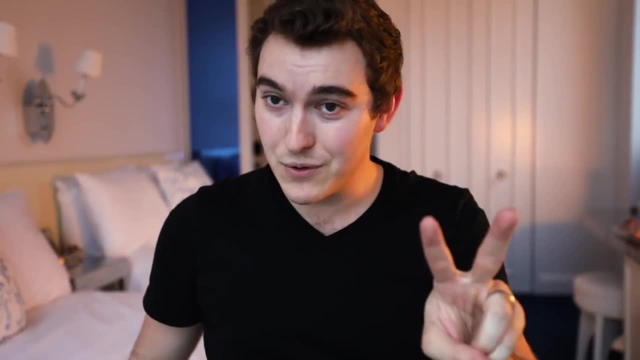 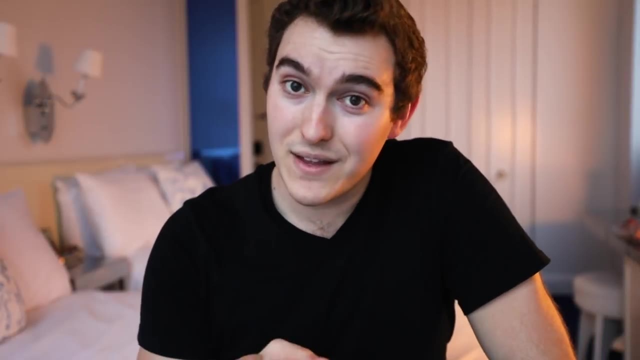 thank you for being a part of the journey. We will talk more about this later. Because, number two, it's almost time for the giveaway. I've mentioned this on Patreon. I've mentioned this on Instagram. I've mentioned this all over the place: 50,000 subscribers. 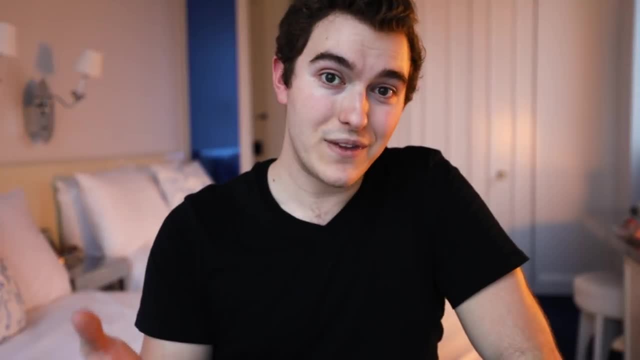 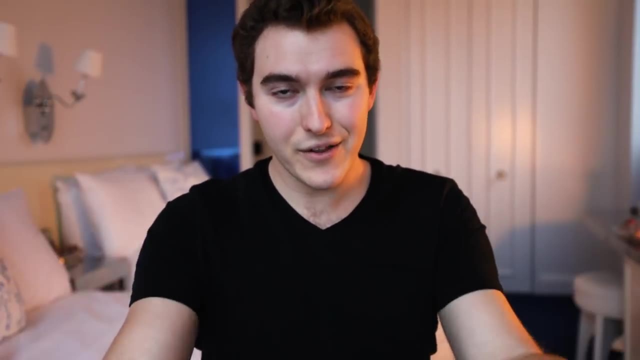 we're doing a giant giveaway. I'll probably make that video very soon. So if you want to be a part of a really super awesome giveaway- my way of showing my appreciation and thanking you guys for all that you've given to me- I want to give back all that I can to you. Make sure you are. 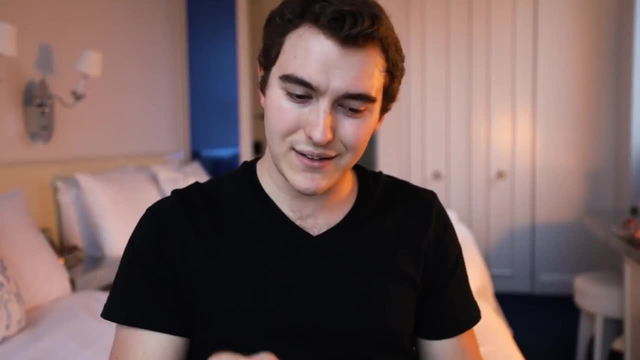 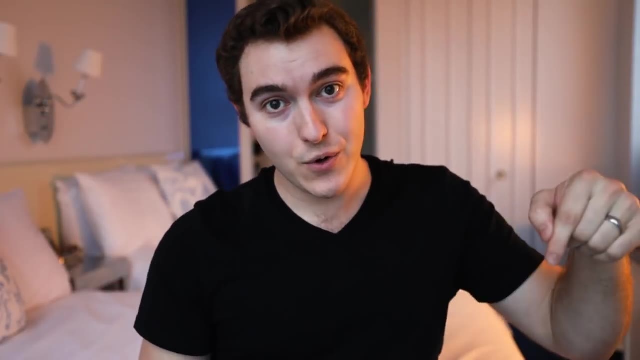 subscribed- if you aren't already- and make sure that you hit the notification bell and tell it that you want to be notified when I post a video. That way you don't miss any of the information. when the giveaway goes live, I will also send reminders on the Discord linked below and also 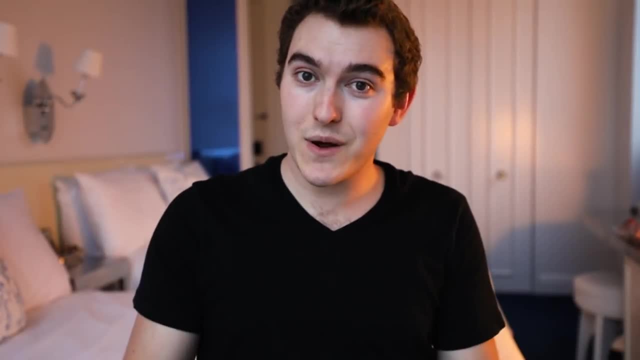 on my Patreon where there's a bunch of other cool benefits Links in the description. Thank you guys for watching. I hope you enjoy Character Animator. I hope you give it a shot. The link is down there as well. And thank you to Adobe for sponsoring this video. Super stoked about it.